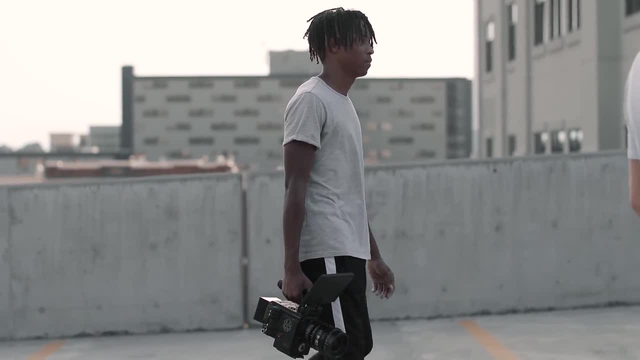 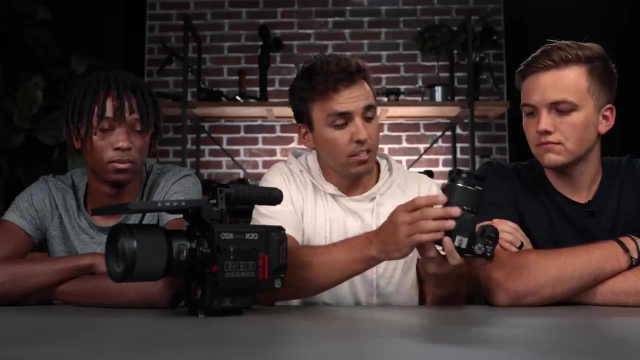 here and see how they compare. Now, Josh has never used a RED camera, so we did have somebody on set just helping him know how to navigate it. but besides that, creatively it's all him. As for Jake, he's just going to be using this little kit lens and a nifty 50 millimeter compared to Josh's. 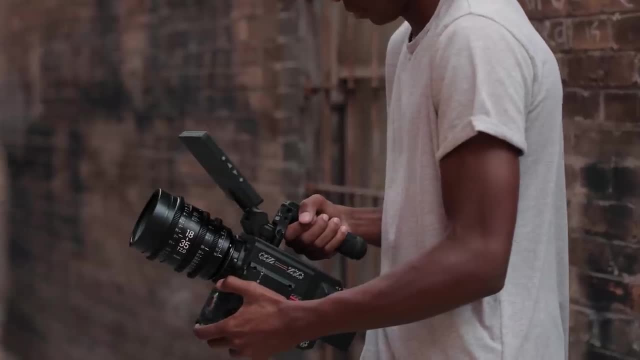 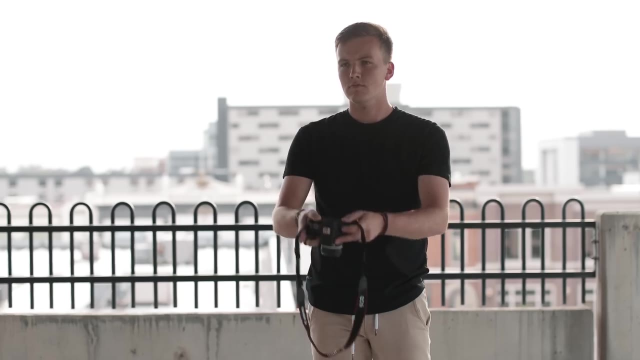 cinema 18 to 35 millimeter lens, so definitely a lot better gear at Josh's hand. but I always tell you guys, it's not the gear that makes the difference, It's the skills behind the camera, and Jake's going to prove that he can produce something awesome with just an entry-level. 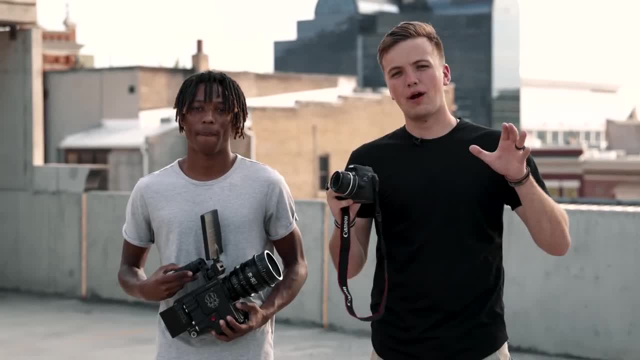 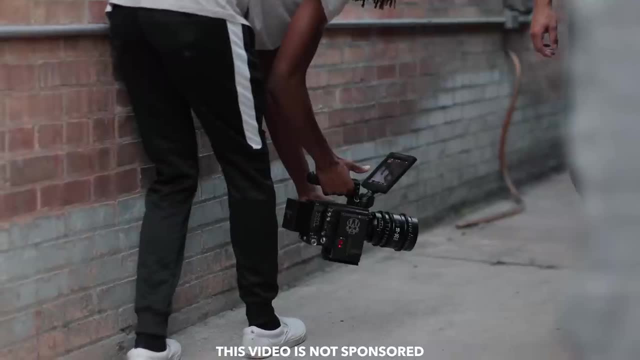 camera, like a lot of you have, So let's get going. All right, so we are now here on set filming. We're going to be shooting our buddy Nate, who is modeling some boots for a company I love. This is a fan-made commercial. They are not paying us to do this and we're going to be taking turns. 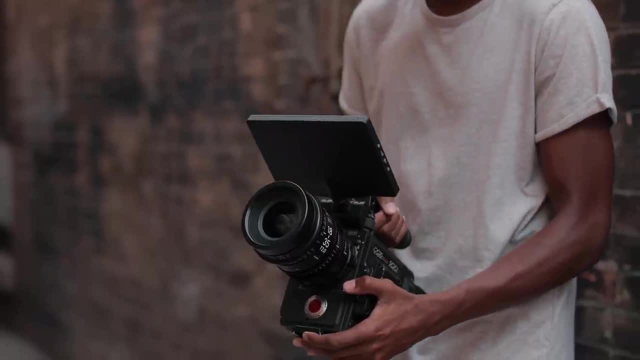 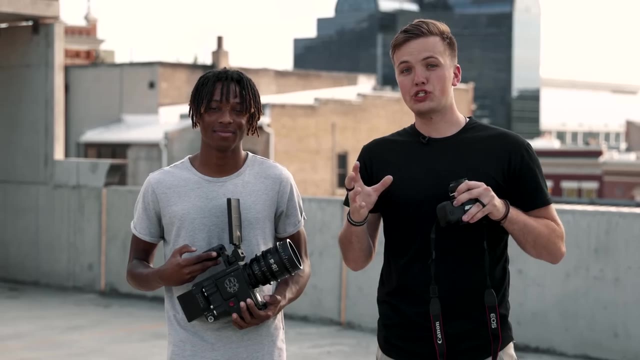 shooting in different locations and seeing what we can come up with as creatives, as storytellers, as cinematographers, and then compare our work after we edit together a small 20 to 30-second commercial- and Josh and I are not going to be shooting together, We don't want to copy each- 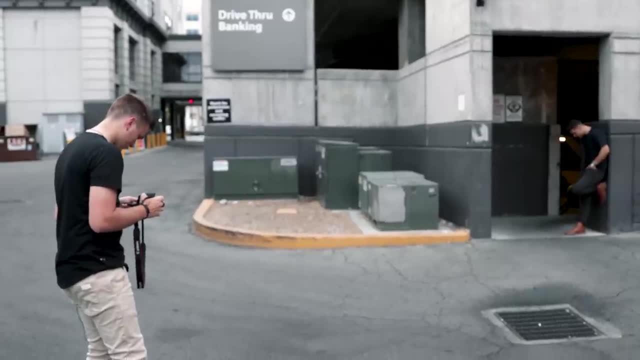 other's ideas. so when I'm filming, Josh will be off set. When Josh is filming, I'll be off set. so that way, as creatives, as storytellers, we're not influenced by each other. So for this first, 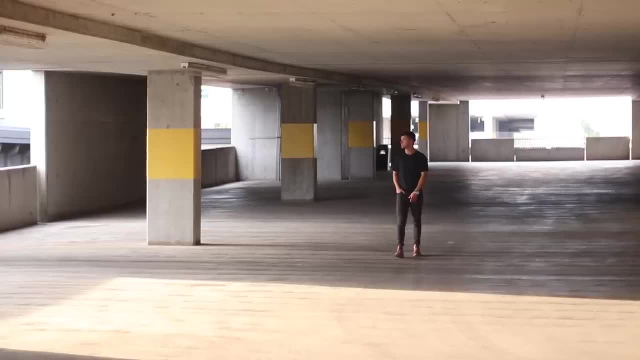 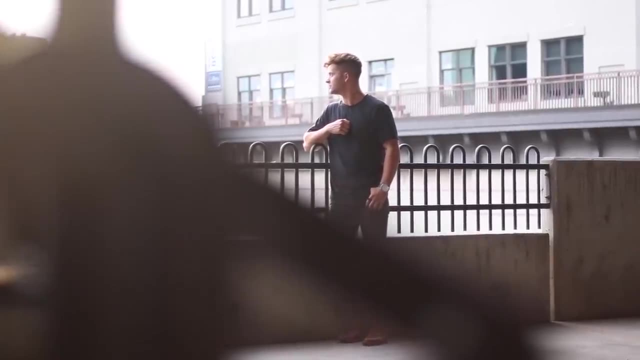 shot. I'm not really sure what storyline I have yet. I just want to get a lot of good product shots of Nate wearing the boot and also kind of just leaving the lifestyle. I want to show someone looking good in the boot and not just show tons of tights of the boot, if that makes sense. 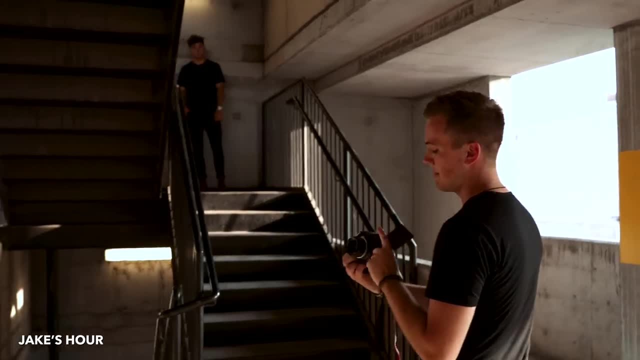 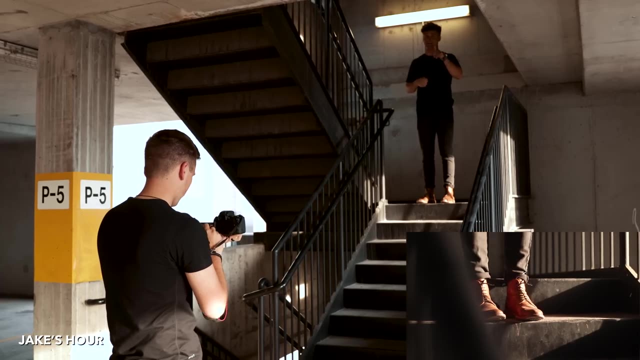 So this is on manual focus as well. The SL2 has autofocus, but I'm using a manual lens so it's going to be a little difficult. Nate, could you step into the sun for me? dude, I want to see what it looks like. Man, this dynamic range is terrible. Pull my focus, hit record. 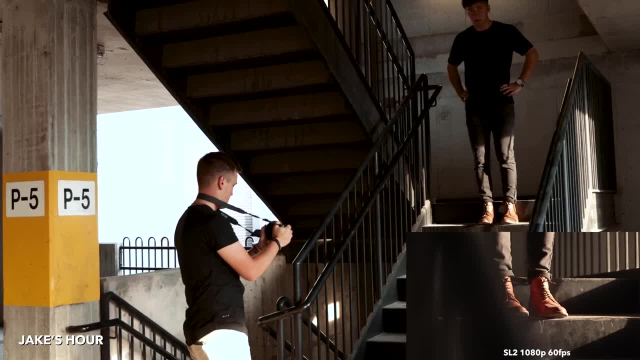 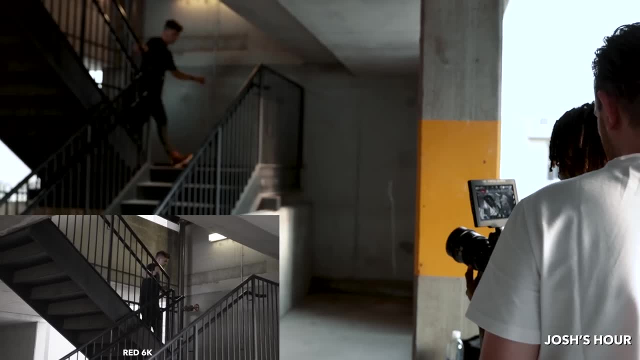 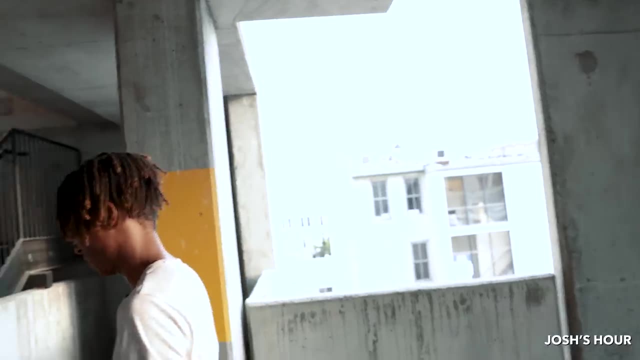 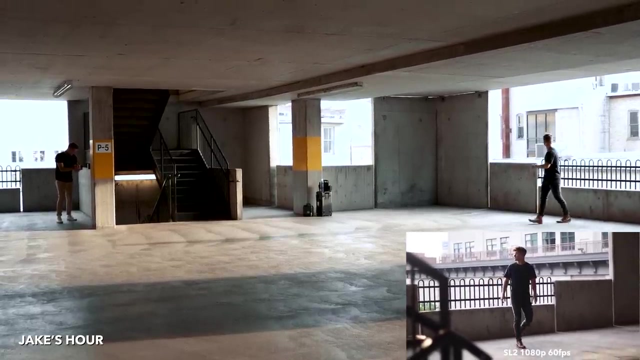 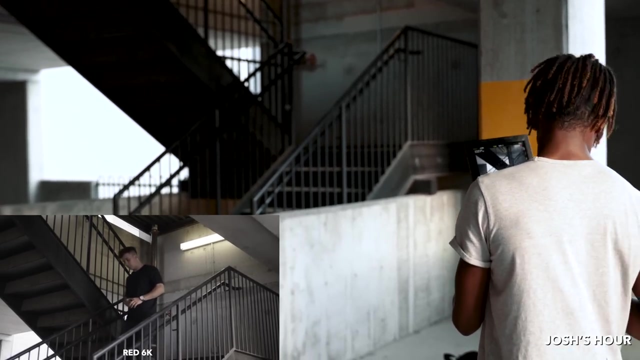 and I'm going to do as stable as I can. Three, two, one go. Oh, shut off, It died on me. Hold on, Yeah, Good thing it died, because I messed up, I forgot to walk up. And three, two, one walking away. Cut, I'm shaking so much. This thing's hard to hold. 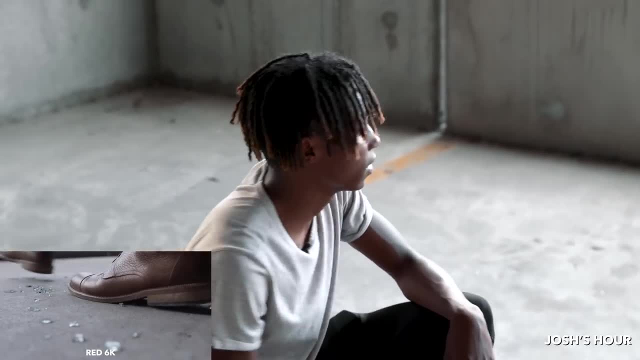 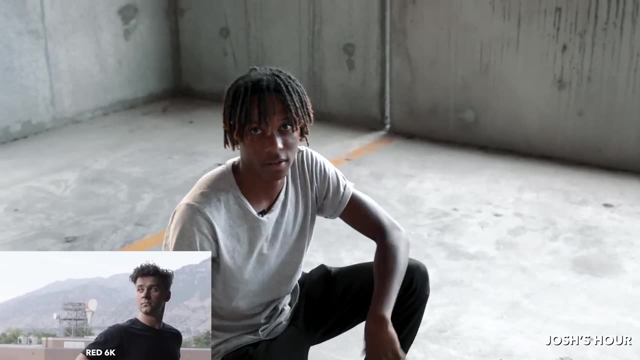 So I want him to like walk through, walking past the glass and then leaning against the fence up there, And then we're going to get another shot of his upper body zooming into like the mountains, and then we're going to end it. I need to do that again, Holy crap. This thing's hard to hold. 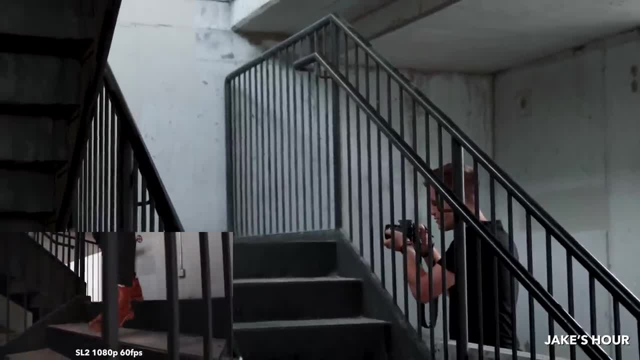 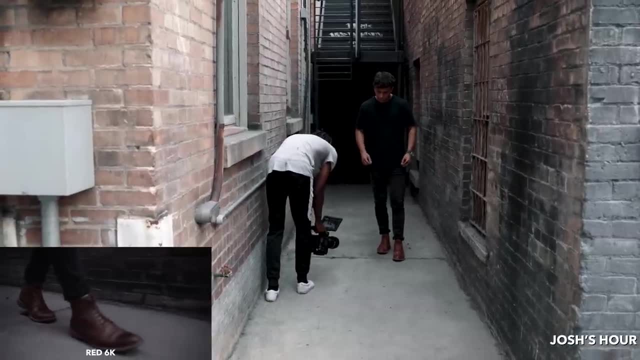 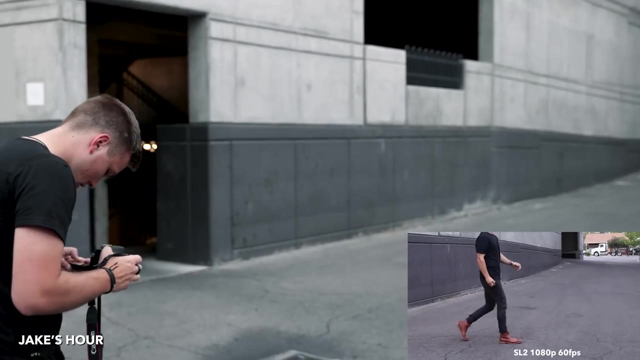 Three, two, one. Action: Nice and slow. Ooh, one more time. That was beautiful, All right. Three, two, one. Oh, I need to redo that. That was bad. All right, We'll call it a day. All right, we just wrapped shooting. I'm a little nervous to. 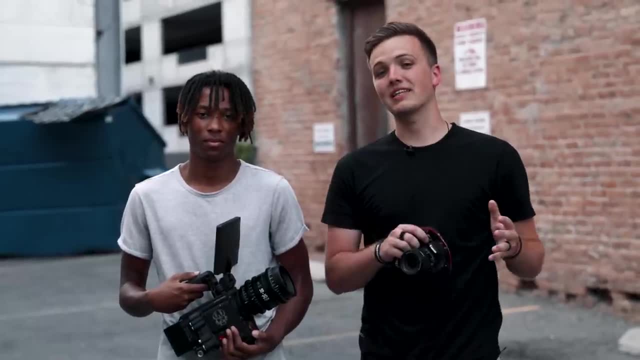 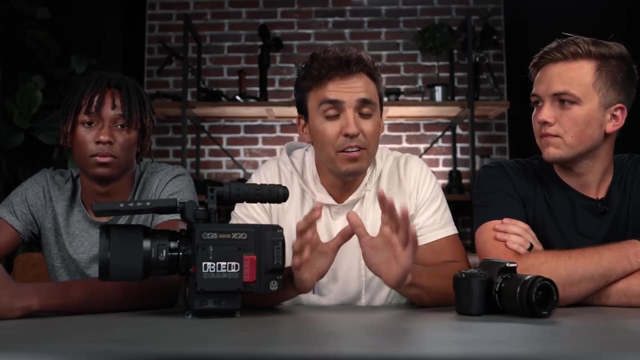 see how my footage turns out. I'm really stoked to see how Josh's footage turns out. We're going to go back into the office, edit together our commercials, watch them with Parker and compare the differences. Here we go And we are back in the office. They have finished their edits and we're now going to watch and 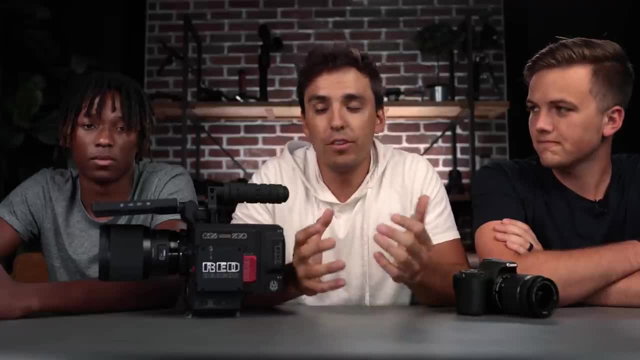 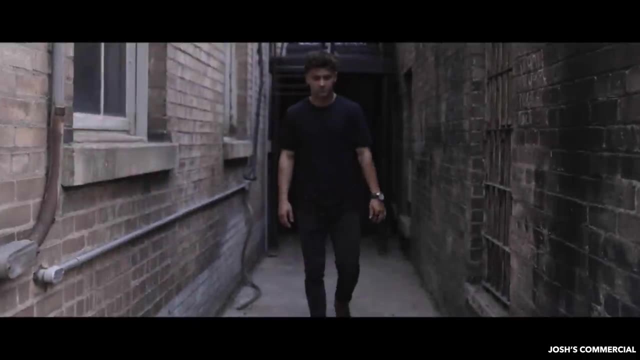 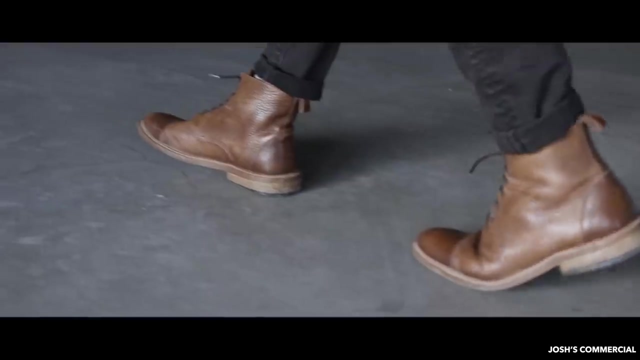 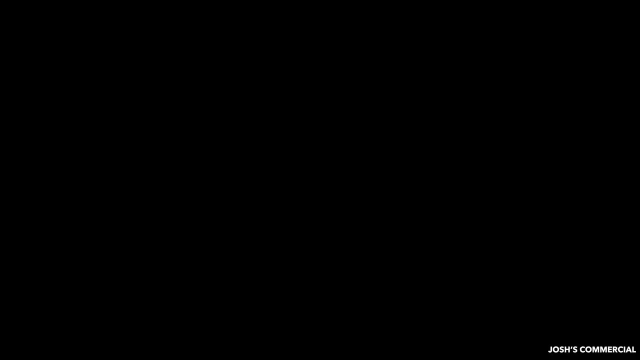 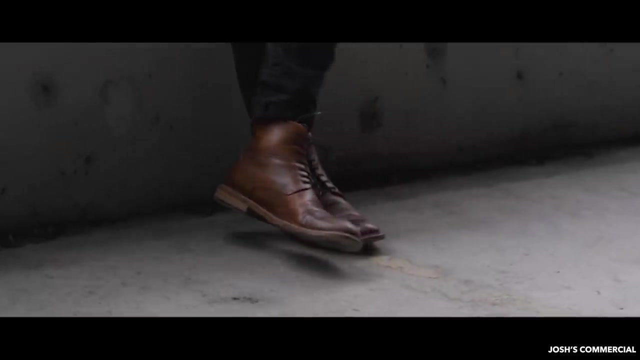 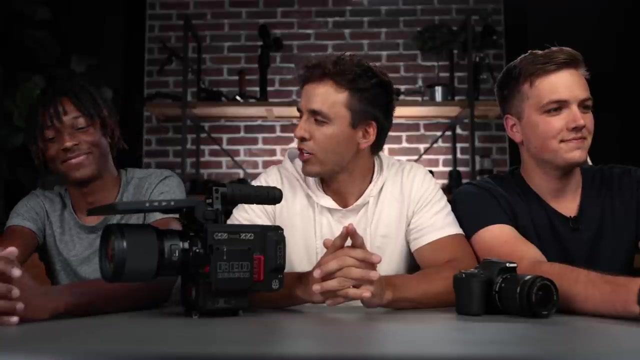 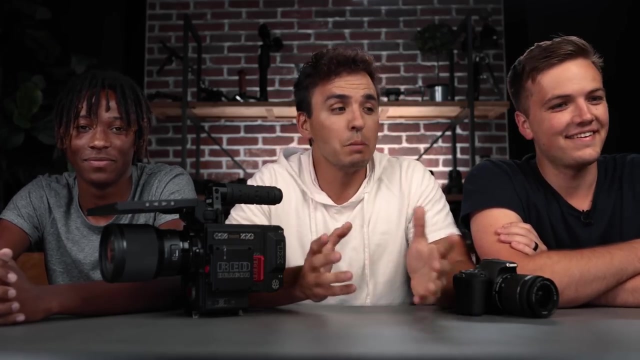 review and give feedback and see how well they each performed with their respective cameras. So first up, let's check out Josh's 30-second commercial. So fight us, Ooh Taft. Nice work, Joshua, Very nice commercial. I am such a proud cousin right there, That is, with five weeks of experience. Like I said before, 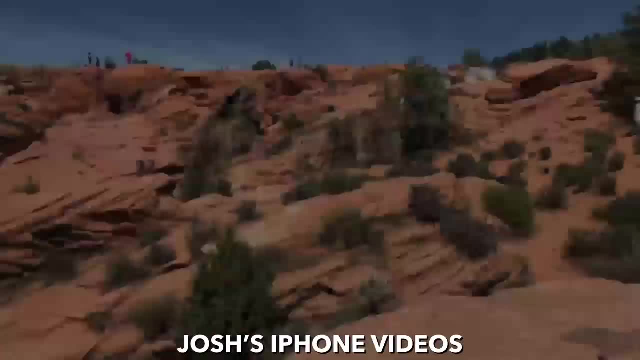 that he would send me iPhone videos and we'll show you some of those videos, like he was shooting just a few weeks ago. Compare that to what he just produced And he's already come a long way. in five weeks We've been training him, mentoring him, talking to him and I hope you'll apply that to those videos. 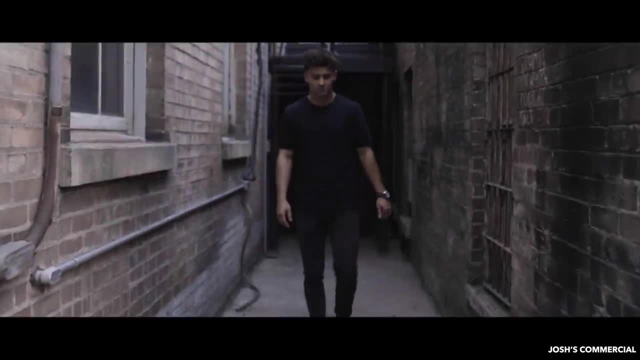 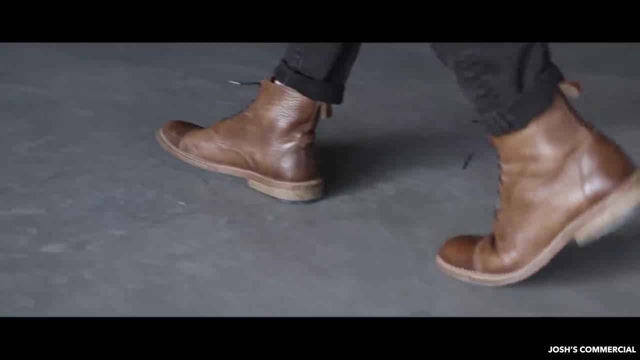 Yeah, I'd totally like to see that come true我 mentoring and helping him grow, So that's better than what you know. just an actual rookie who's not shot anything ever would produce. So awesome job, Josh. You can see just from having good gear. 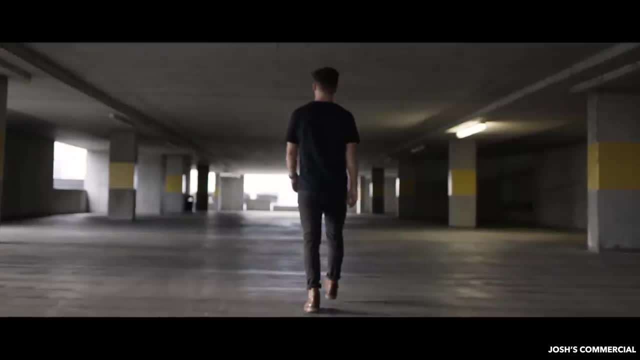 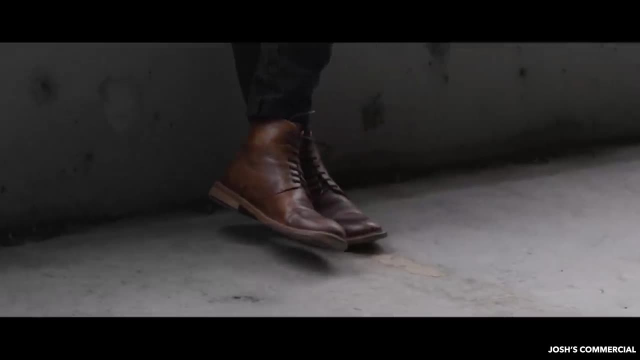 that does make a difference, Like you really can produce quality stuff just by having some nice gear, even if you have never used it and don't have a ton of experience. So that's something to keep in mind: that gear does make a difference. It doesn't make all the difference, I don't think it. 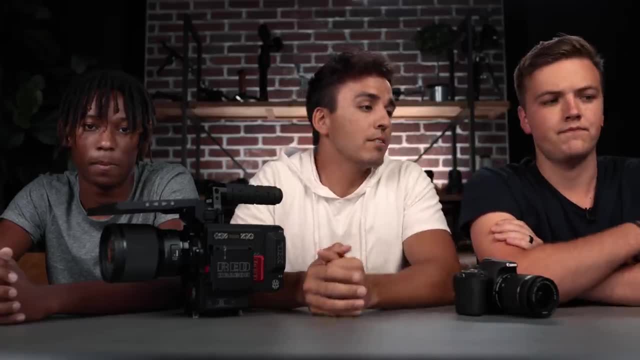 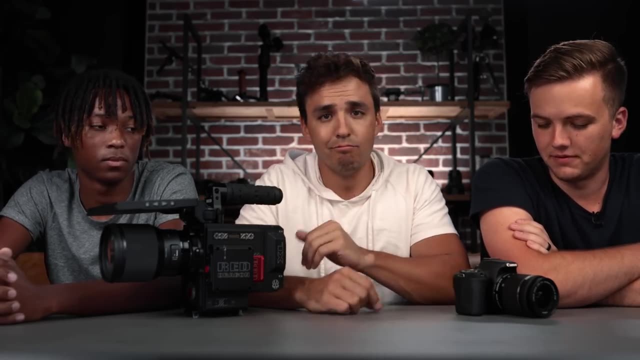 makes most of the difference, but it does make a difference. But let's now watch Jake's. see how that compares with a nice Canon SL2.. By the way, that was shot in 6K and this is going to be in 1080.. So see if you can even tell. 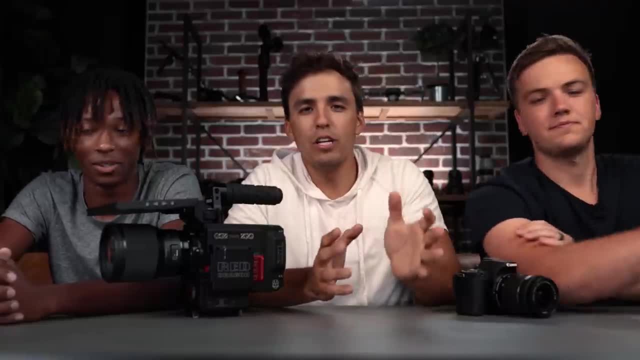 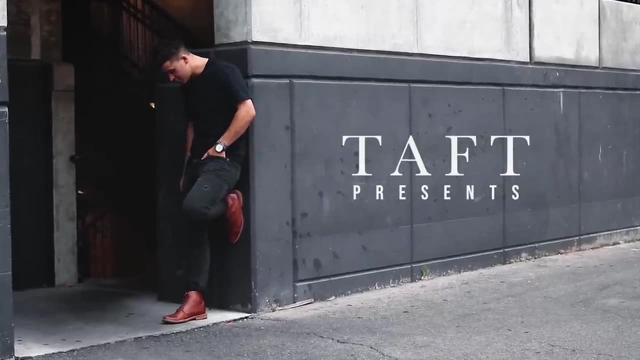 Loved it. I was when he showed me that I was like you really shot that in the SL2? I mean, that is a $600 camera and that is a commercial that could pass and that you could charge thousands of dollars for, And that just testifies to how important it is to have experience. He has five. 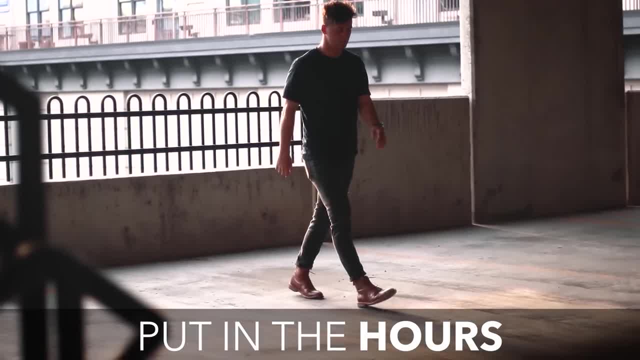 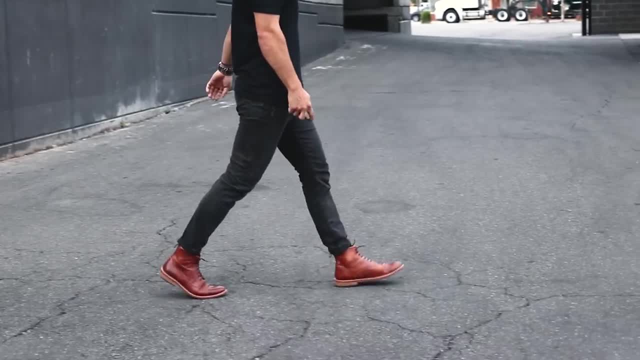 years of experience, He's probably put in 10,000 hours. Like I always tell you guys, you got to put in those hours, those repetitions. I was just telling Josh the other day: I'm like man, if you want to be a professional, if you want to be able to do this full time, you just got to put in hours. 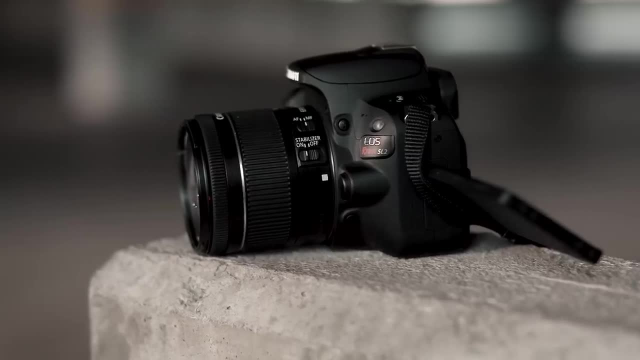 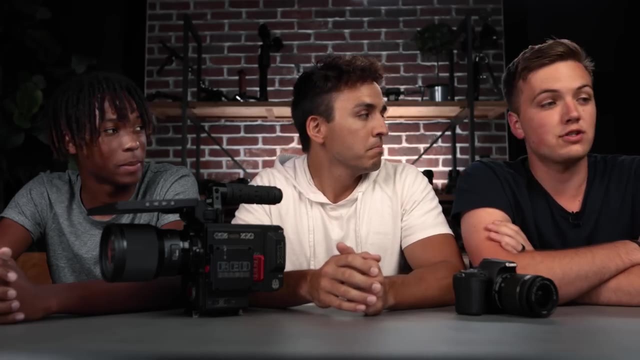 And Jake has done that, And so when you throw at him a entry-level camera, he's still able to produce high quality results. Now, what did you guys think of those two? watching them back to back, What were your thoughts? First off, I had to put a lot in post to make that look even better. 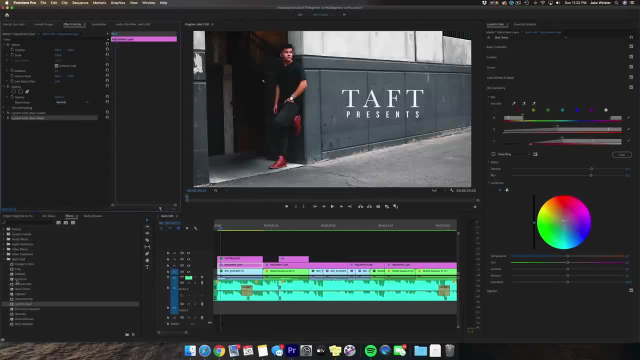 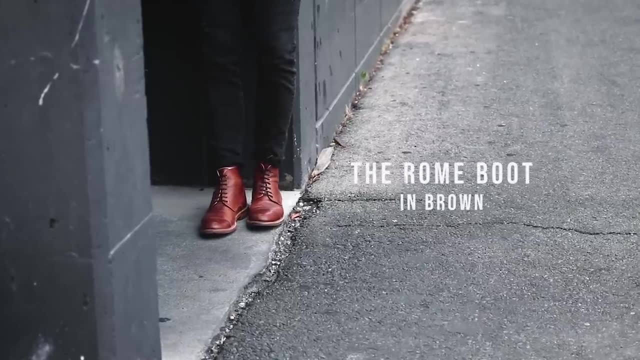 I had layers of color correction. I'll show you kind of some of the layers I was adding, some of the sharpening I was adding. I did warp stabilizer to everything because I was shooting handheld And so a lot went into the post-production side to make it look just as good as I possibly. 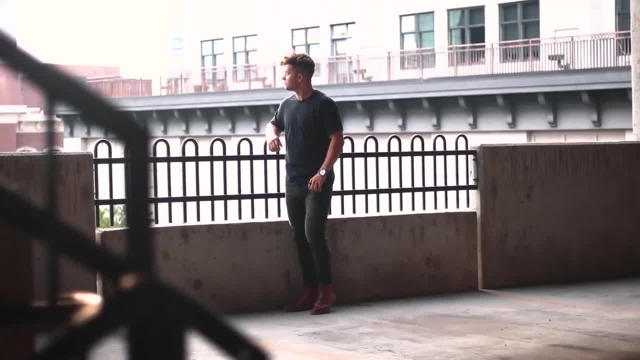 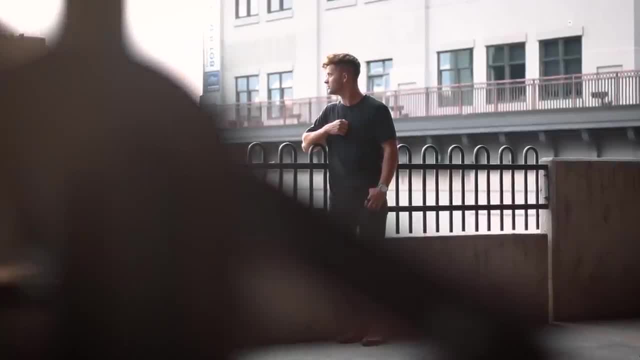 can to compete with a red over here. But I think I think some of the key differences it's just: it's just knowing, like Parker said, just what experience can teach you that gear can't teach you. And that's some shots to get some angles, to get some depth to create. 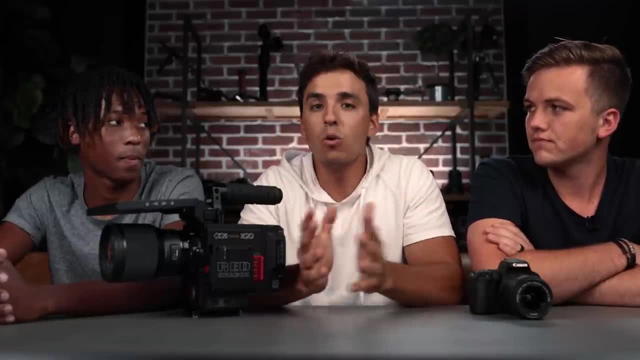 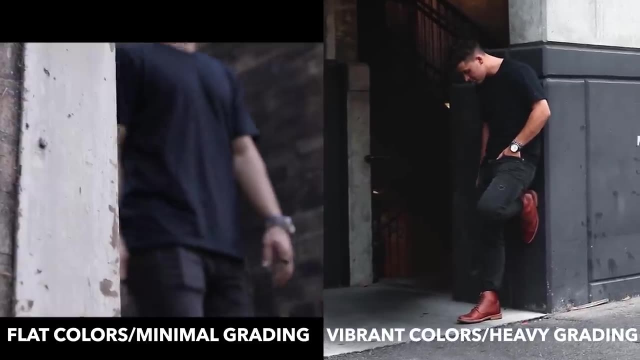 things like that. As you can see, like Josh's came quite a ways just by having gear, But what really stood out to me with Jake's is the colors. Josh doesn't have a ton of experience color correcting or color grading And so his image looked pretty flat, and this is a pretty flat. 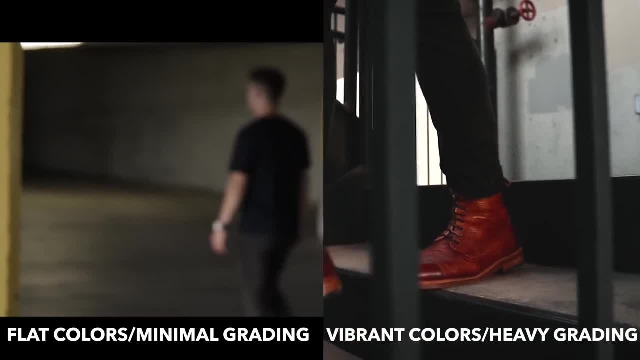 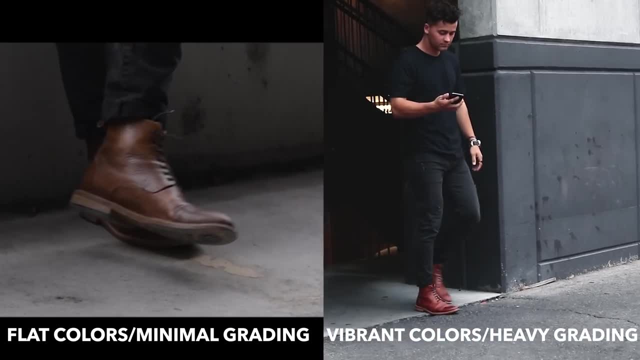 camera. It shoots in raw And so if you don't know what you're doing in post then you really can't manipulate that image and get the most out of it. As far as color grading goes, the colors just popped. on this It just looked more like a professional commercial, whereas this looked 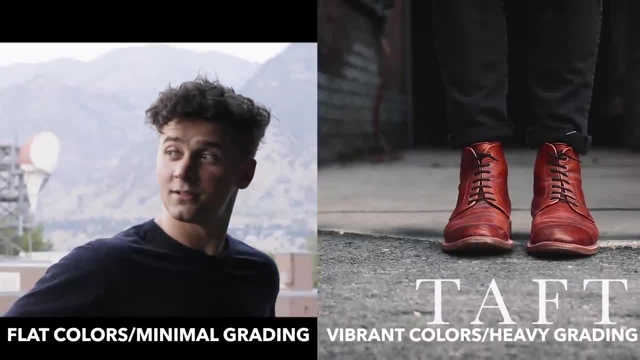 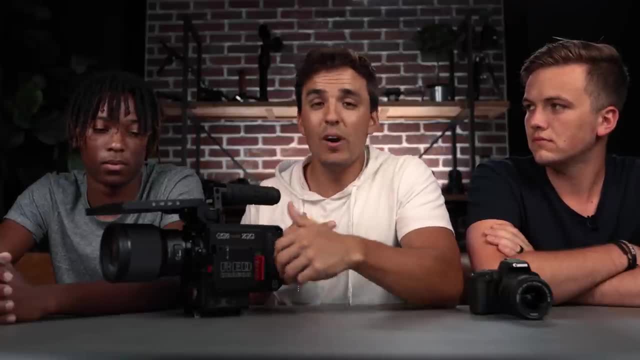 like a first draft where we hadn't quite done the color correction yet. And that just comes down to experience And anybody who would be given a red without knowing how to use it or how to color grade it. that's how anyone would look, And so Josh did the best he could, with what knowledge he. 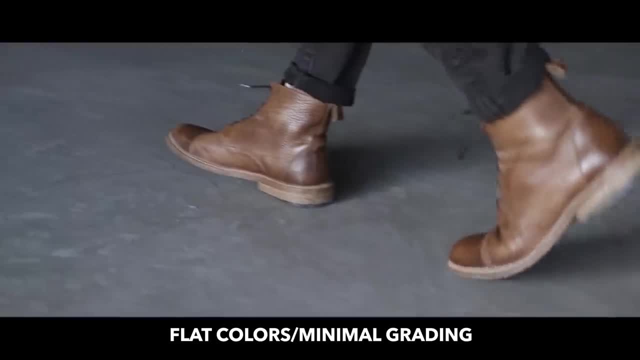 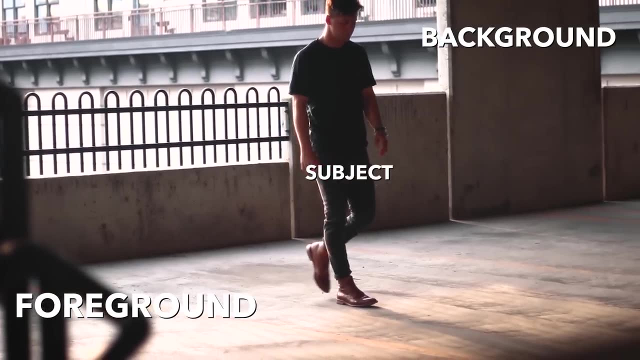 had, But that was the biggest thing that stood out to me immediately were the colors just popped off the screen with Jake's Another thing with shot selection, like Jake mentioned, Jake just has a lot more experience with creating depth and getting different angles And you just notice a. 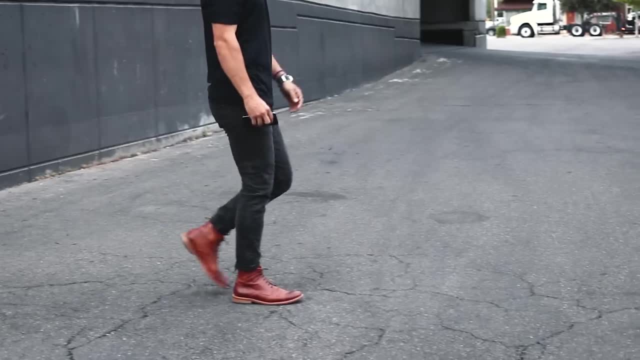 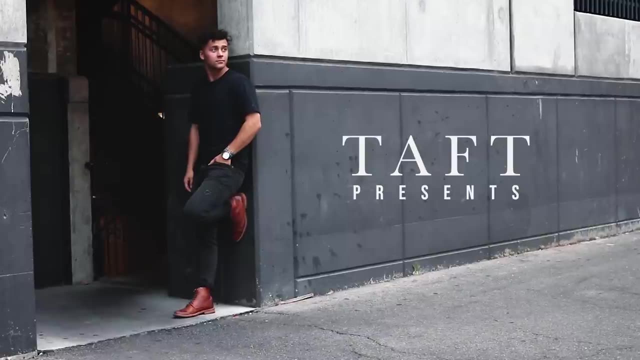 different level of cinematicness with Jake's shots that he's getting, where he's creating more depth, He's using foreground a little bit better And, as far as the effectiveness of the commercial itself, you notice that Jake is using titles to describe what we're looking at. He focused a little bit. 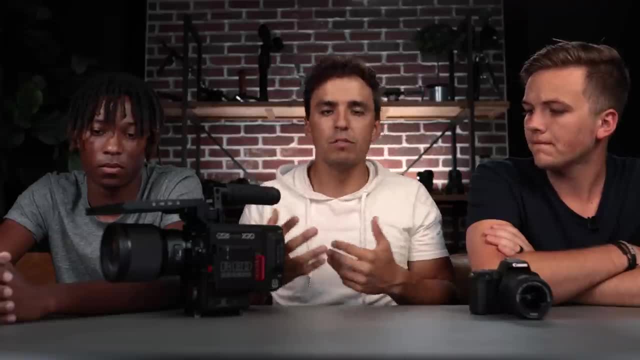 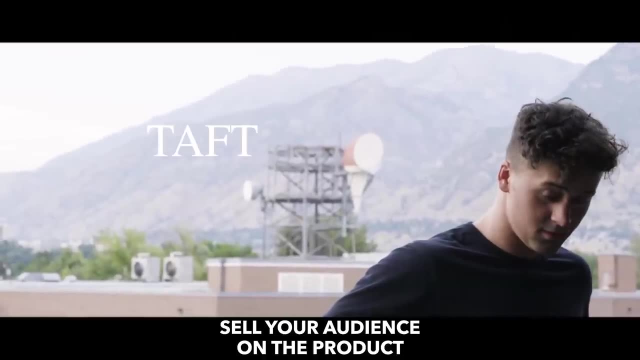 better on the boots, whereas you know Josh is just kind of grabbing shots of his model walking around and it's not super focused on the boots, And that's something. once you've worked with a client and done a bunch of product videos, you just start to learn what types of shots your client 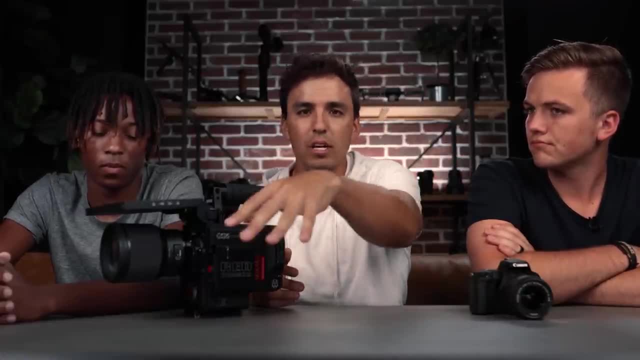 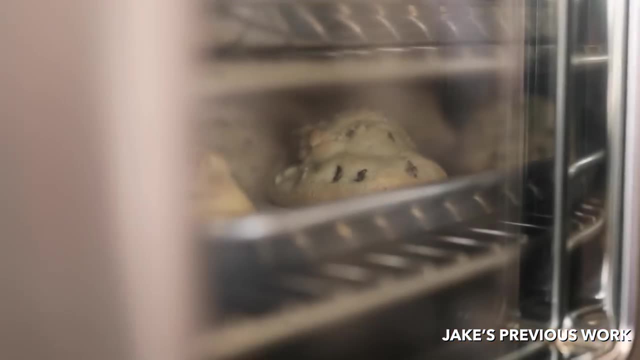 is going to like and which ones they throw out and say, yeah, I didn't like that. one can replace that with something else And Jake's done so many of these He's, he's gotten that feedback and he knows I shouldn't get a shot like that because they're going to ask for something different. 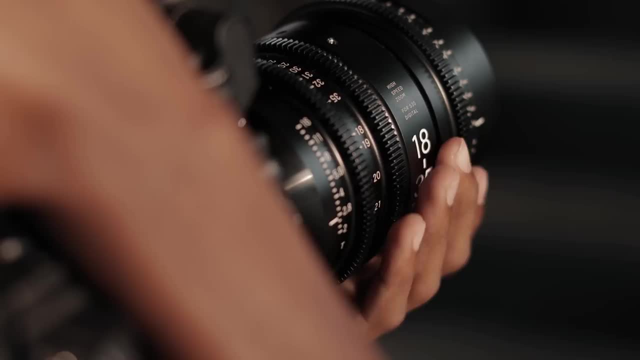 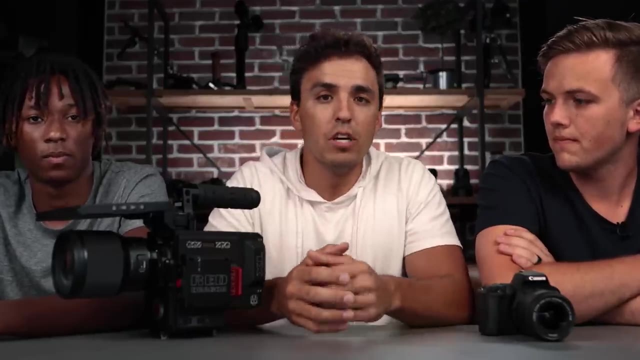 Whereas Josh, he's never shot for a client yet And so he's just filming whatever he thinks is going to look good but doesn't have the perspective of a client- Again, someone that just comes with experience. One of the thing I noticed was just nailing focus. There's a few shots I noticed where 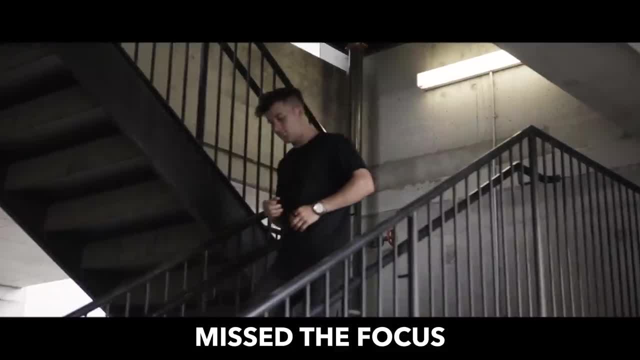 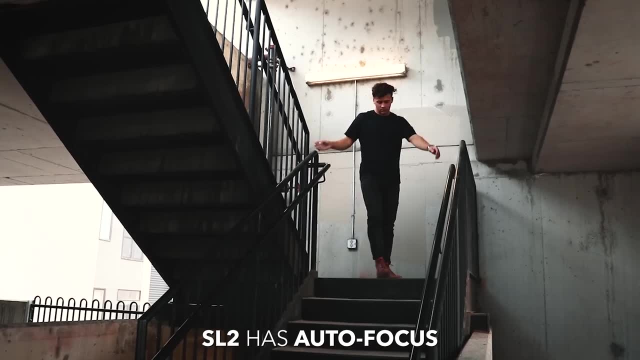 Josh was a little bit out of focus And again that just comes down to experience of knowing how to use the camera. So that was one advantage Jake had was his camera had autofocus versus this one is all manual. So if you don't know how to use manual focus really well, that becomes a 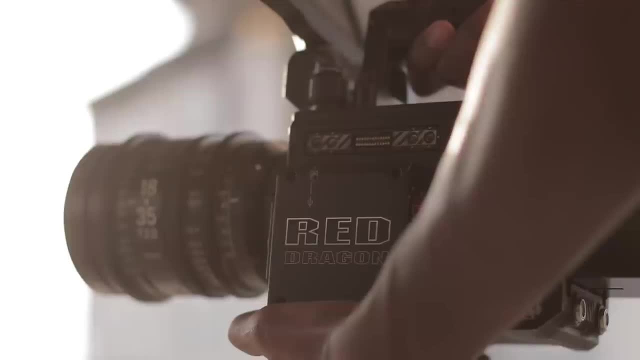 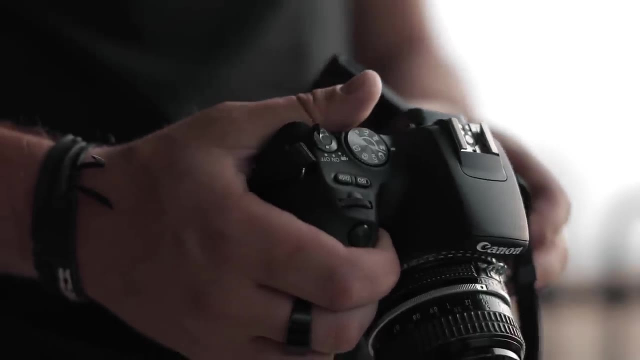 disadvantage. And so these big cinema cameras, as nice as they are, they still have some drawbacks that you guys shooting on some of these cheaper cameras you got to realize and take advantage of those And those can really help you out in areas that someone with a cinema camera might struggle. 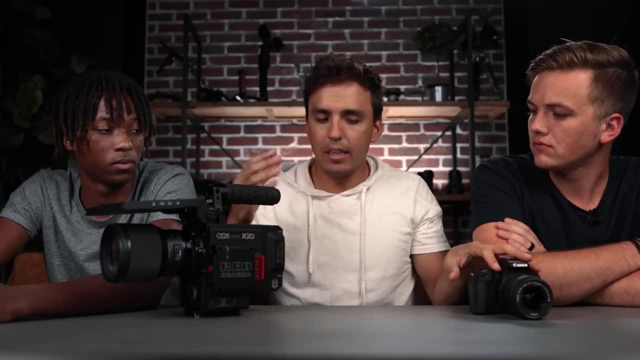 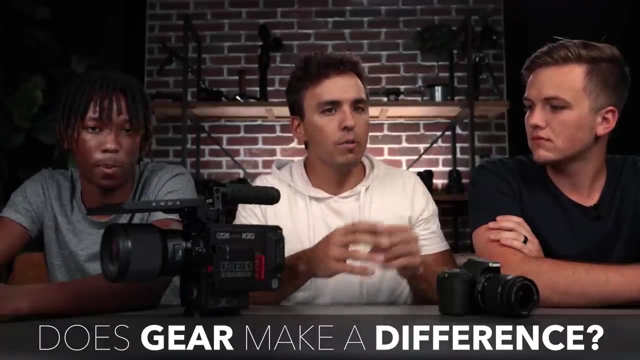 to practice that manual pulling focus And so, as you guys can see, like this was a fun comparison for us just to be able to see how much does the gear actually make a difference. And, as you can see from that, personally I thought that you can do just as much professional work as you can with. 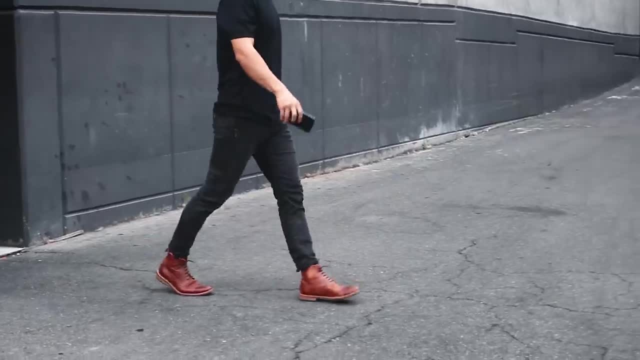 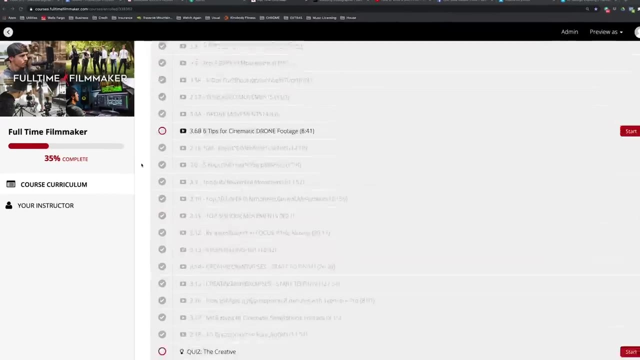 the red if you know how to use the gear And that's what we teach inside a full time filmmaker. the ultimate online film school highly recommend you guys checking that out. We have mentors here to help you guys. we have over 400 tutorials that's going to teach you guys how to get the most out of